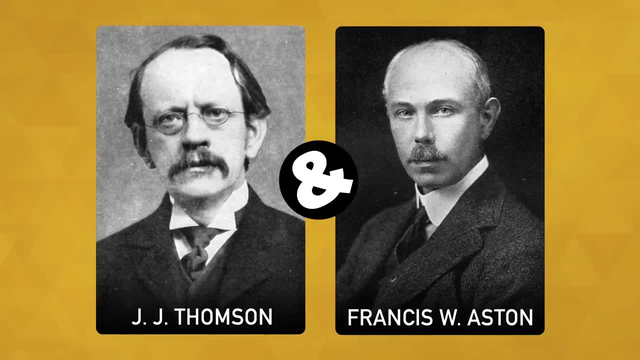 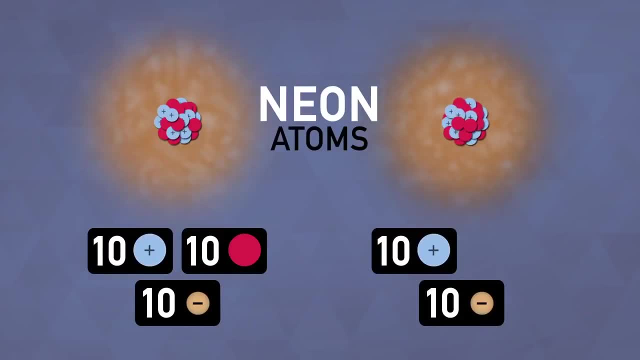 his student, Francis W Aston, identified two different types of neon atoms: One type with 10 protons, 10 electrons and 10 neutrons, And then one with 10 protons, 10 electrons and 12 neutrons. Aston went on to invent a groundbreaking machine that he called a. 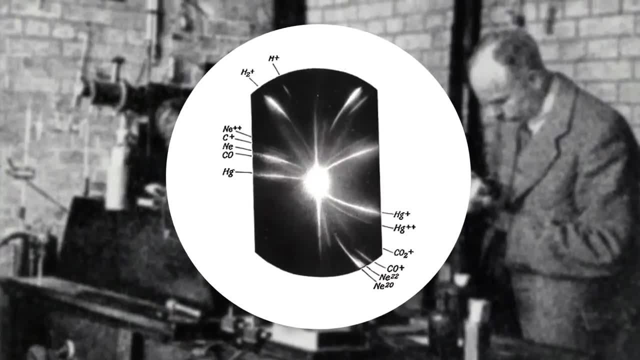 mass spectrograph. Using this machine, Aston identified hundreds of other isotopes of other elements. The Mass Spectrometer is now used in labs all over the world. So this is another union of the two massive spectrograph. It uses the mass spectrograph asery. 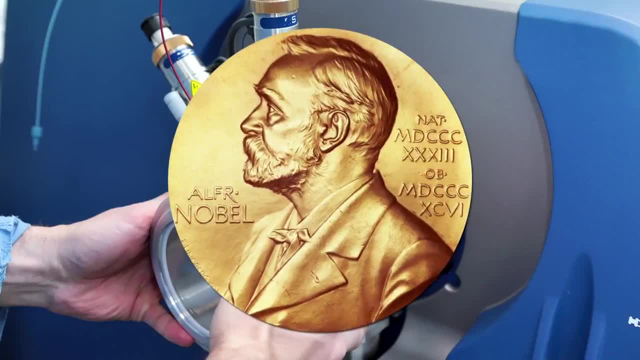 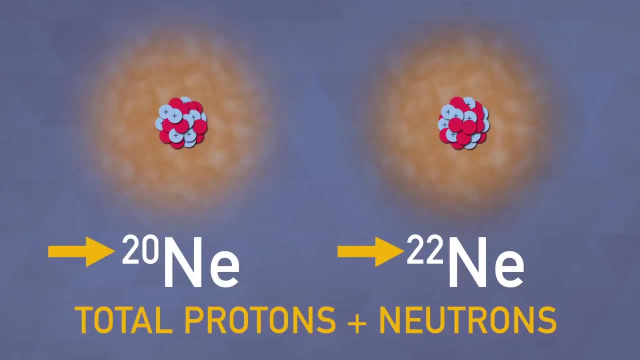 and Aston won the 1922 Nobel Prize in Chemistry for his work. These are the isotopes of neon that Thompson and Aston saw. The numbers you see here tell you the total number of protons plus neutrons in each atom, and they also tell you the isotope's approximate mass. 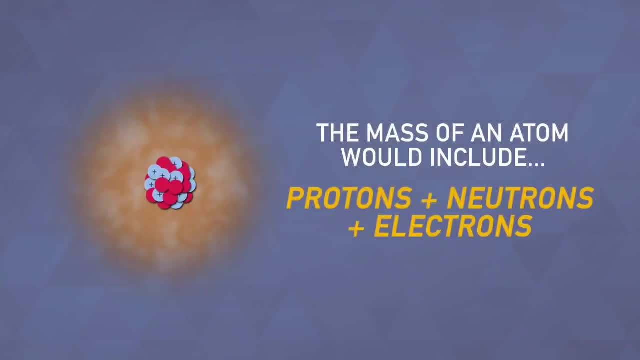 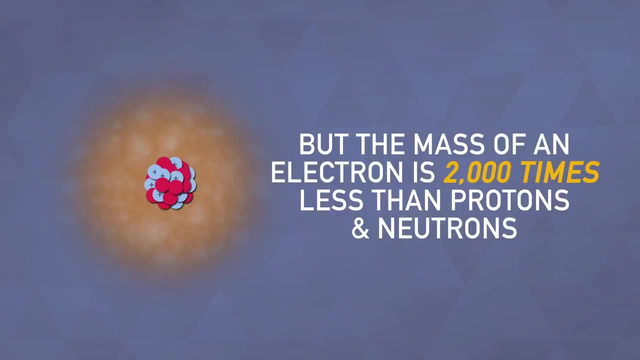 Technically, the mass of an atom would include protons, neutrons and electrons, but since the mass of an electron is almost 2,000 times less than that of protons and neutrons, we can basically ignore them. When it comes to atoms and their behavior, there's an important distinction to make. 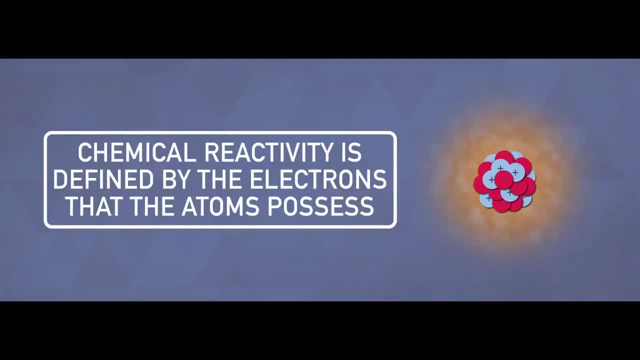 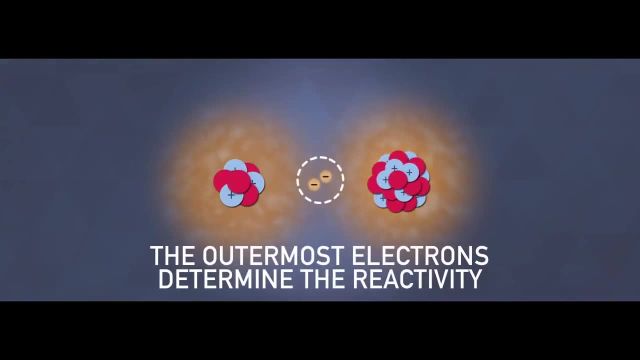 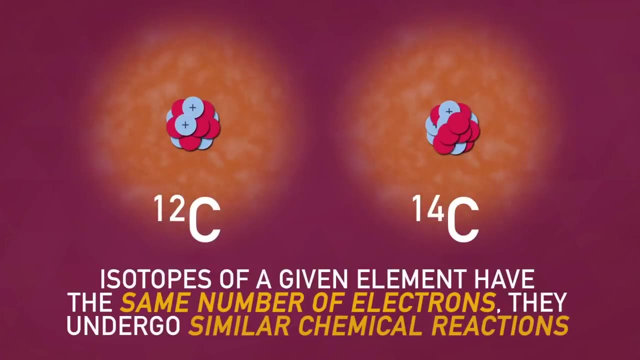 between chemical reactions and nuclear reactions. Chemical reactivity is defined by the electrons that atoms possess. When atoms come into contact with one another, it's their outer electrons that interact and determine the type and the intensity of the reaction. Since isotopes of a given element have the same number of electrons they will undergo. 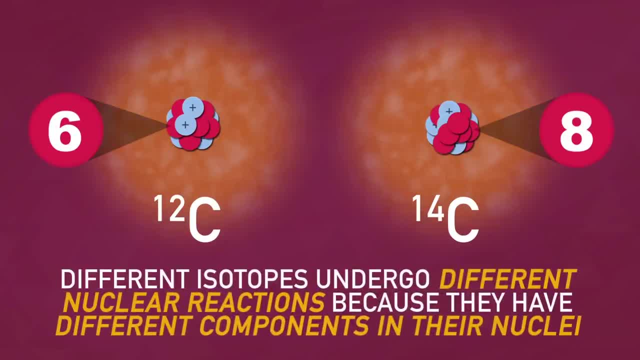 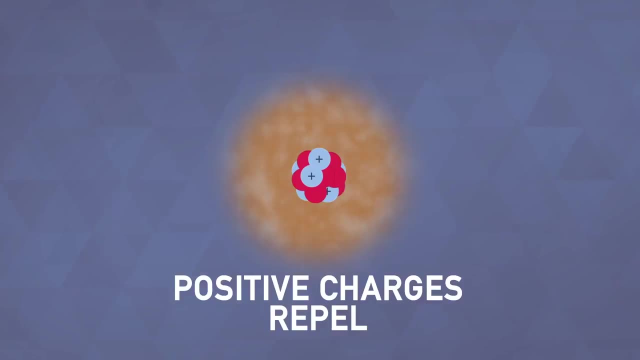 similar reactions. On the other hand, nuclear reactions rely on the particles in the nucleus, so different isotopes will undergo different reactions. So what happens in a nuclear reaction? Basically, something changes in the nucleus, Because the nucleus is made up of protons and neutrons. you might think that all of 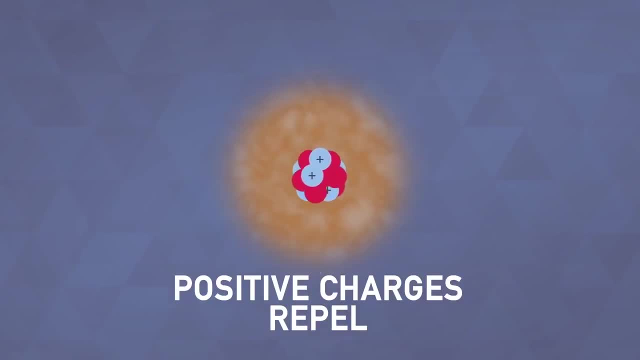 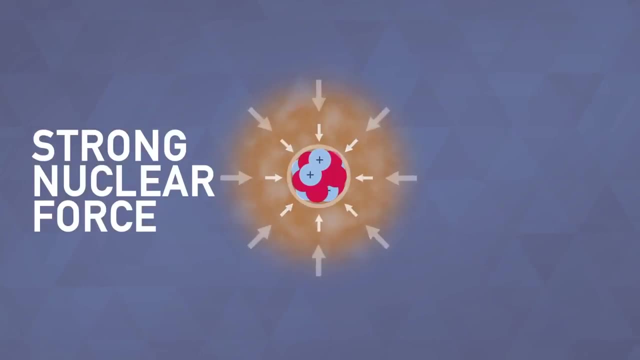 those positive charges crammed together and repelling one another would make the nucleus unstable. Luckily there's a force known as the strong nuclear force that acts as the glue that holds the whole thing together. But when the nucleus of an atom contains lots of protons and neutrons, or when certain neutron-to-proton 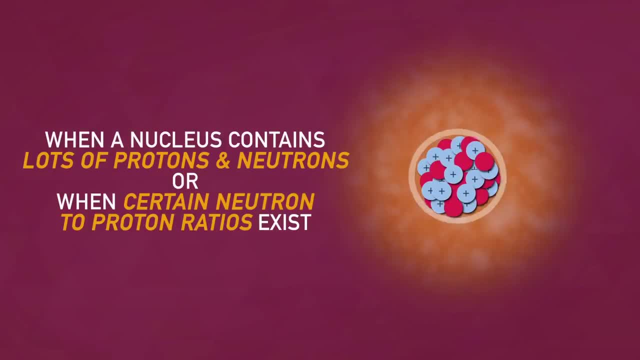 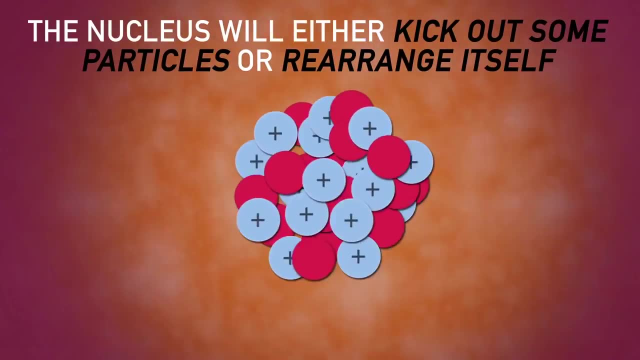 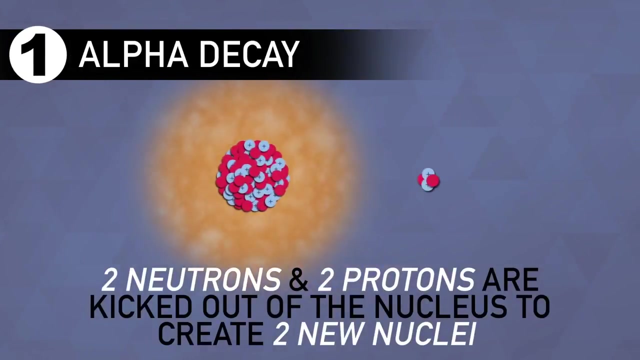 ratios exist. even the strong nuclear force can't hold it all together and the whole thing can become unstable. When that happens, the atom's nucleus will either kick out some particles or rearrange itself. Typically, one of three things happens. Alpha decay is when two neutrons and two protons are kicked out of the nucleus to form two.